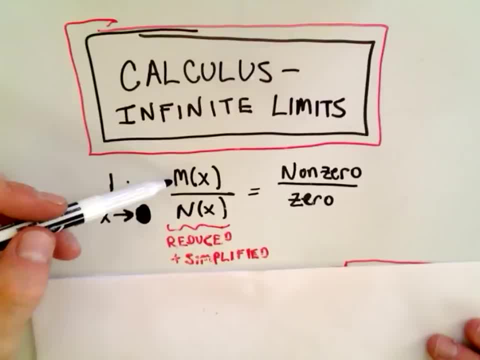 Whatever it is down here. So we've got a limit, We've got some function of x and another function of x, And let's assume that it's reduced and simplified And suppose what happens is we calculate our upper limit to be something non-zero, And our bottom limit, though, will approach zero Again as x approaches whatever. 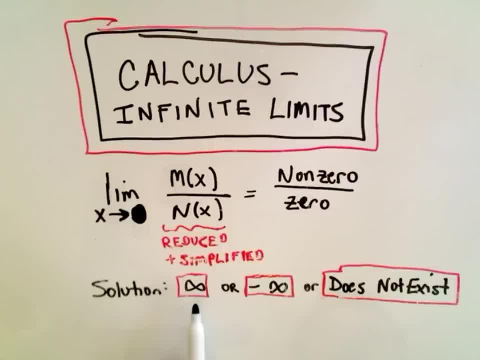 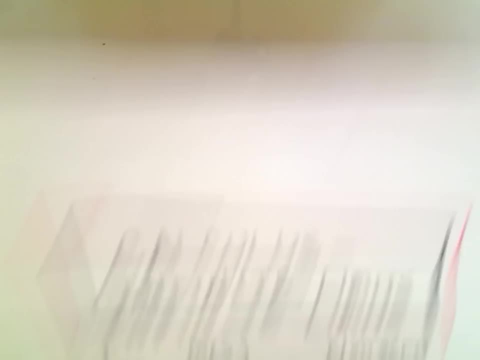 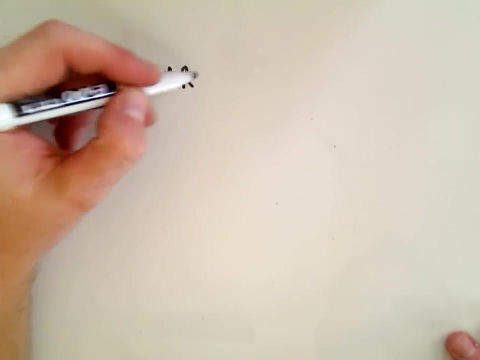 So, typically, what's going to happen? your solution is going to be one of these three things: Either it's going to be positive infinity, Negative infinity, Or the limit will not exist. I say typically. I would like to say always it'll be one of these. I'm trying to remember if there's some, I don't, I just I don't, I don't see how it could happen. Maybe I'm missing some little, something very obvious. Okay, the first thing, before I actually calculate a limit is I just want to make a little remark, And maybe for some of you it's very obvious, But I've asked enough people to where it's not. 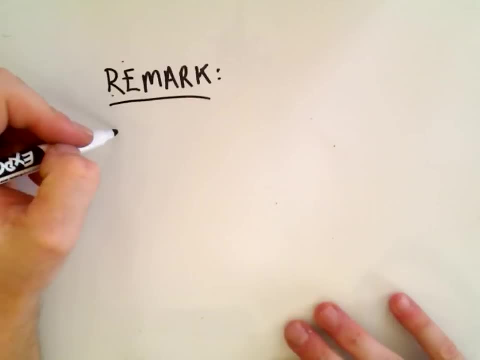 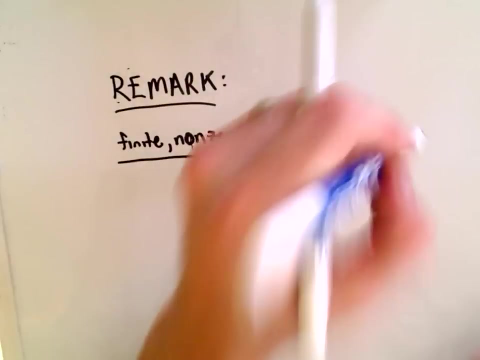 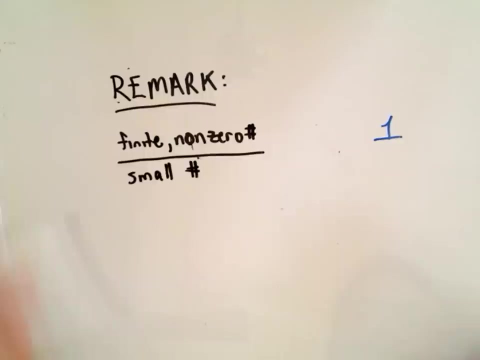 Okay, so suppose we take some finite number- Finite, I should say non-zero- number. Okay, so suppose we have some finite, non-zero number. How about, like one? And suppose we divide this by a small number. What type of number are you going to get out? That's the basic question. 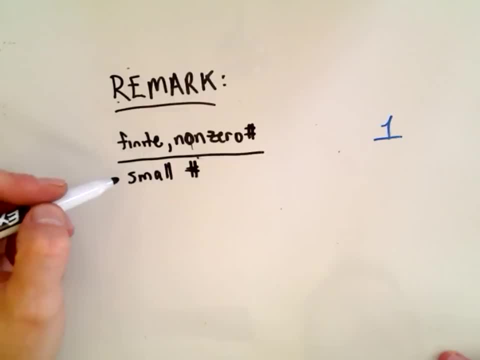 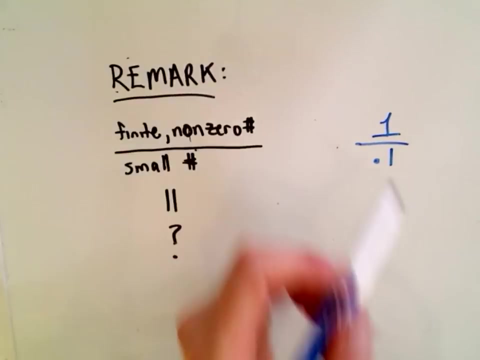 So a finite, non-zero number Over some small number. It could be positive, It could be negative. Well, let's just do a couple examples here, real, real quick. I mean, think about one divided by .1.. For us people in USA think about it as being you know how many dimes, .1, 10 cents go into a dollar, Well, 10.. Suppose we divide that finite number by something even smaller, Say .01.. Okay, how many pennies are in a dollar? 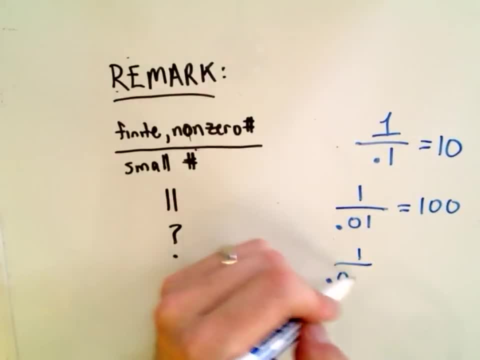 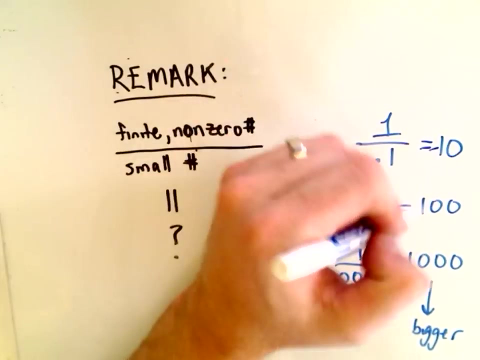 Well, there's a hundred, There's a hundred, And so on and so forth. Divided by .001, I'm going to get 1,000.. So notice, as the number on the denominator, in the denominator, gets smaller, the number on the right-hand side is getting bigger. And if the number that I was dividing by was negative, negative, negative, of course, it would just make it a big- I say big in quotations- it would be a big negative number. 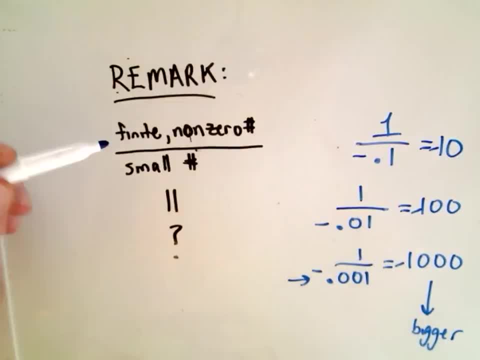 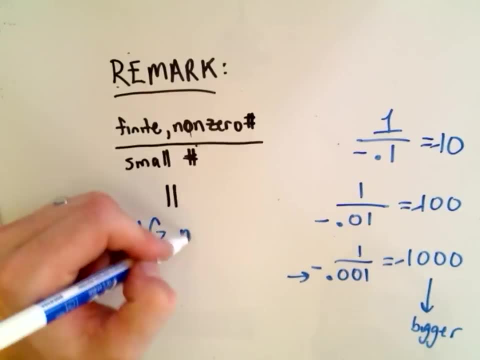 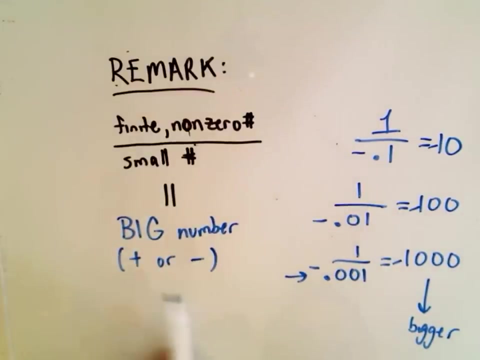 Okay, so the idea is a finite, non-zero number over a small positive number is going to be a big number, Okay, and depending, it's either going to be positive or negative. obviously That you'll have to think about a little bit. okay So, but this is the basic, the fundamental idea on these limits. 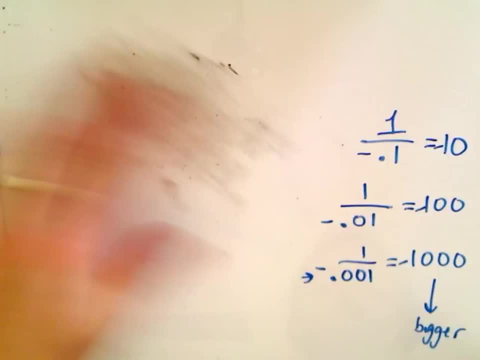 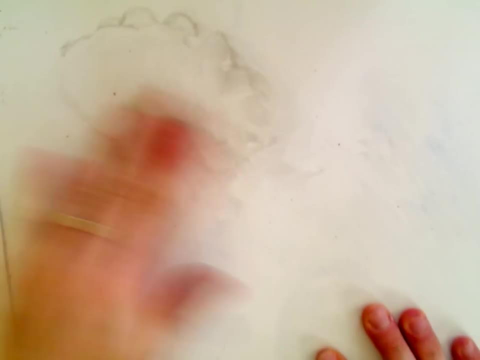 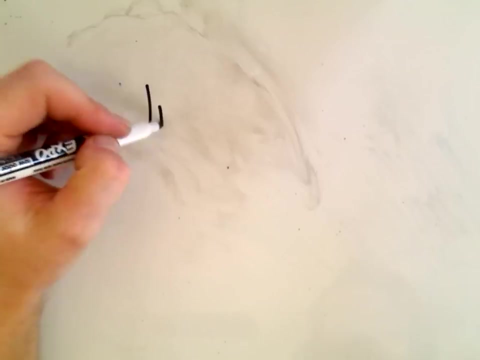 So let's actually do a couple problems. I don't know where my paper went to clean this board off, So it's going to be a little dirty. it looks like, Suppose we're calculating the limit as x approaches positive 5 from the right of 6 divided by x minus 5.. 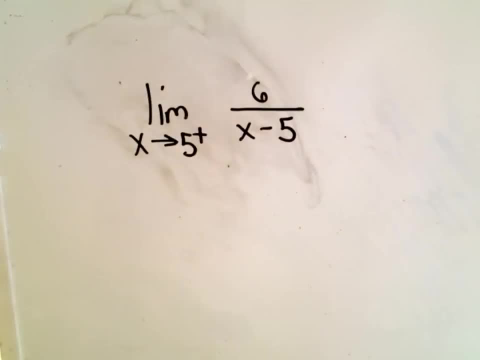 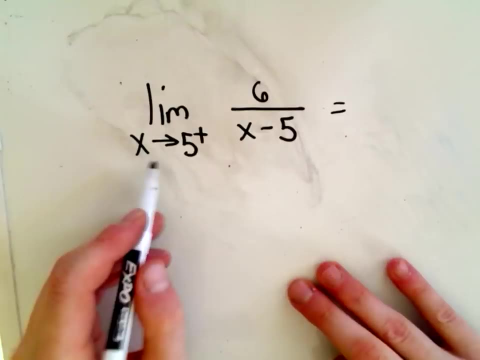 Okay, so the first thing that typically you do with limits is you try to plug the value in And evaluate it. Okay, so in this case, if we plug in 5, and again it's approaching 5, remember the plus means this. plus means from the right. 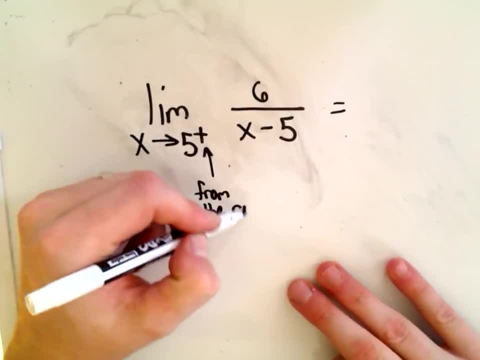 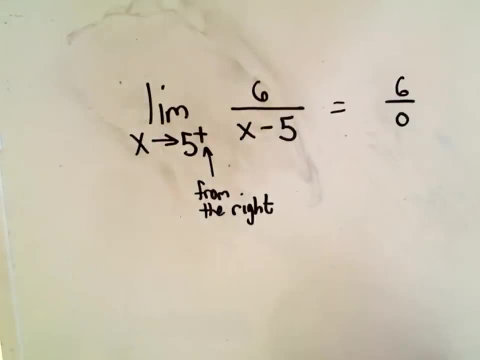 So just a little bit bigger than 5.. So if I take a number, if I were to plug 5 in notice, I would get 6 over 0, which is undefined. So that's the problem. But- and this is how I basically evaluate them, 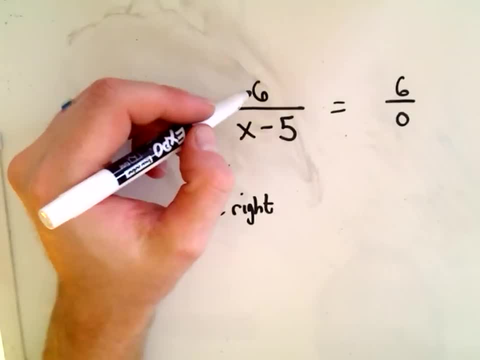 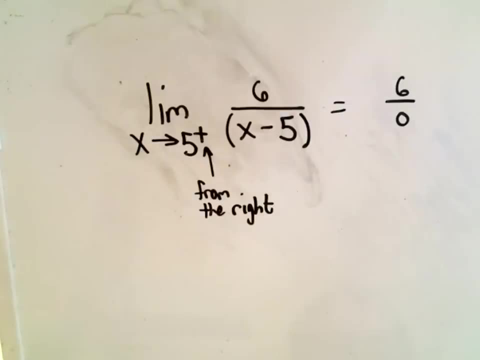 So any place where I get something non-zero, it's going to be negative. So any place where I get something non-zero, that's fine. The places where I get something that's zero out, those are the places that I stop and I think about those a little bit more. 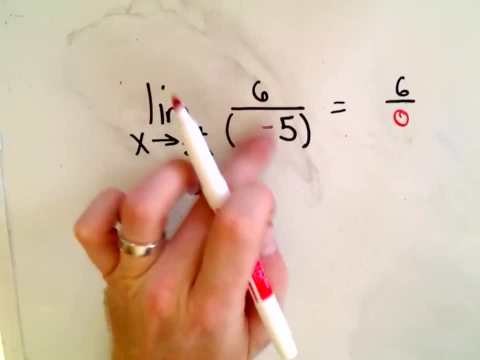 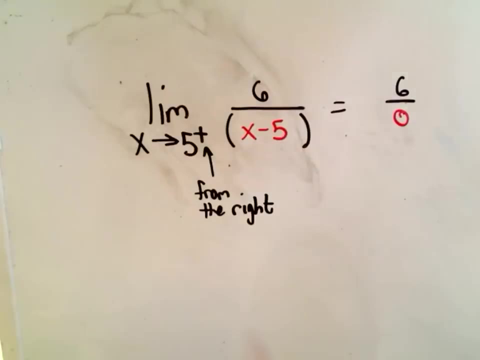 So notice, we're going to get a zero for the x minus 5 part. So to me that's kind of the critical part. That's what I'm worried about. Well, what's going to happen as x approaches 5 from the right? 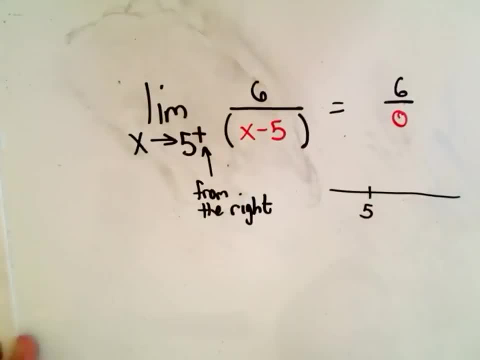 Well, here's the number 5.. So if we're approaching it from the right hand side, we're going to get an x minus 5.. Okay, So this is going to be negative. So if we're approaching it from the right hand side, we're going to get an x minus 5.. 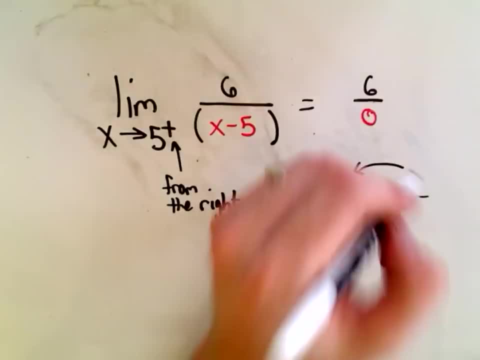 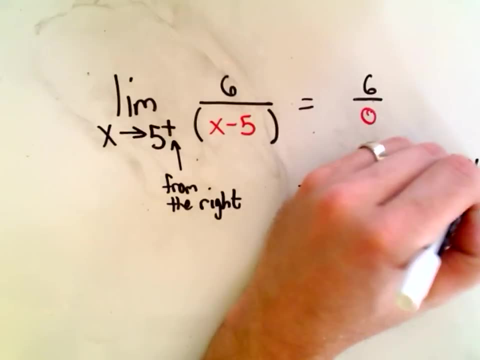 Okay, So this is going to be negative. That means we're taking numbers bigger than 5, so 5.1, 5.01, 5.001.. So we're getting closer and closer to the number 5, right. 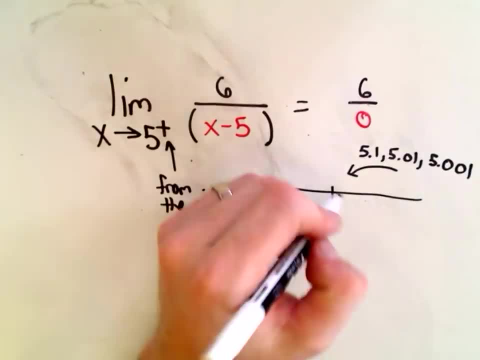 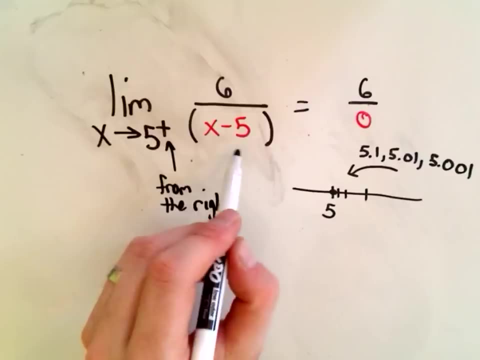 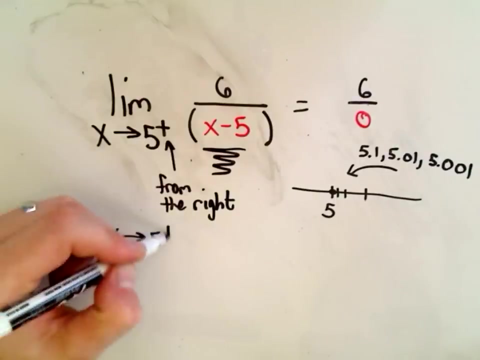 My numbers are getting smaller. They're approaching 5, so 5.1, 5.01, 5.001.. If I were to plug those into the denominator, what would happen? Well, as x approaches 5 from the right, I think you can see what's going to happen. 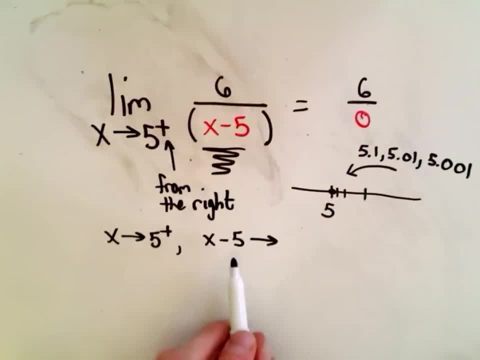 The quantity x minus 5, it's going to get closer to 0, because the numbers themselves are getting closer to 5.. When I subtract away 5, it gets closer to 0.. But notice, is it going to be bigger than 0 or smaller than 0?? 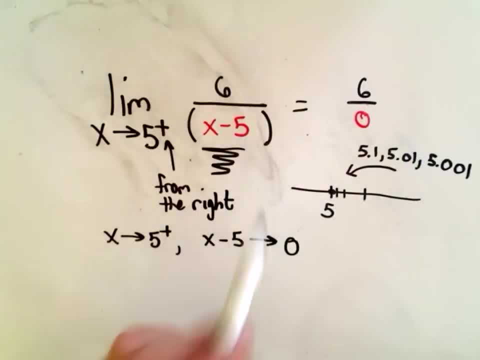 Well, since the numbers themselves are bigger than 5, when I subtract 5, they're going to be bigger than 0. So that means I'm approaching 0.. I'm approaching 0 from the right. Basically, it's definitely not correct terminology. 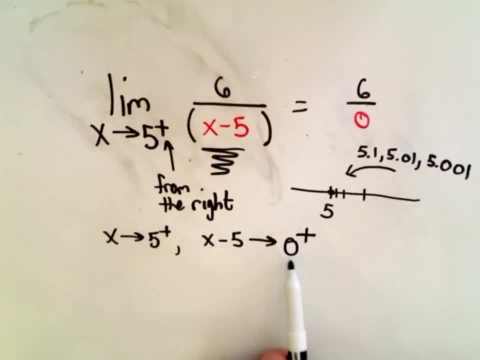 I think in my head it's like having positive 0.. It's arbitrarily close to 0, but it's a positive number. So what I do when I do these problems is I think about the 0 on the bottom as being positive 0.. 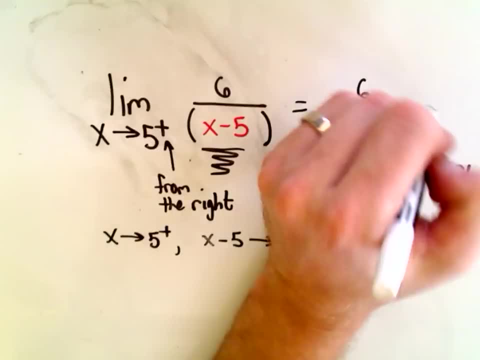 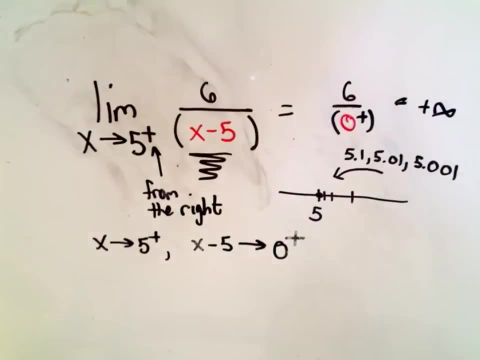 So when I see a number divided by 0, that to me is infinity, And then I just think about signs. So on top it's positive, on the bottom it's positive, so it's going to approach- It's positive- infinity. and that's my answer. 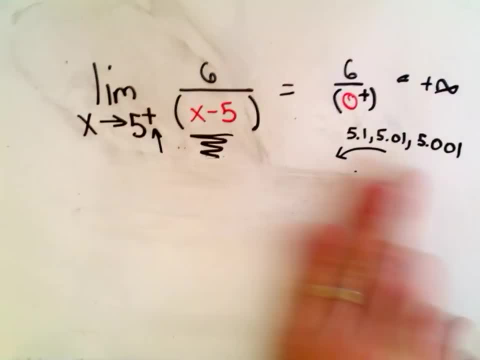 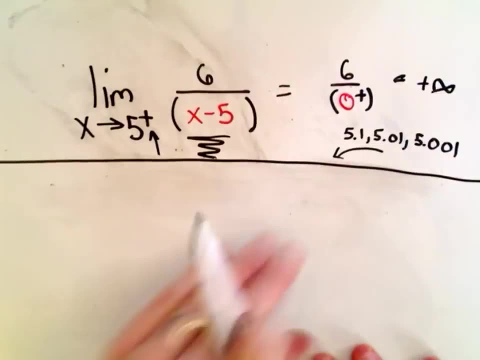 Okay, so maybe let me do another one of these here. Sorry, I guess I should go get something and clean this off and remake it, but I could make two videos in that time, Okay, so let's do another limit problem. Let's do one a little harder. 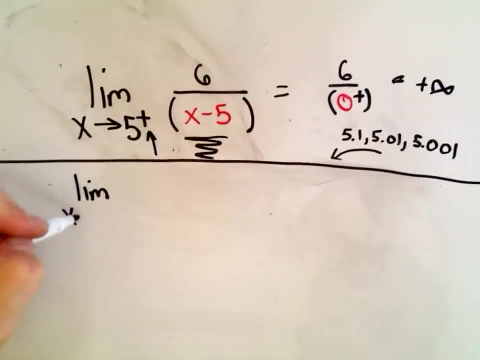 Suppose it's the limit as x approaches 0.. I have x minus 1 divided by the quantity x squared times x plus 2.. Okay, and I want to take the limit as x approaches 0 of this, So forget all about my earlier one. 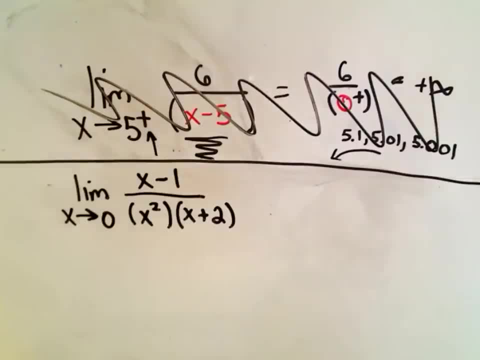 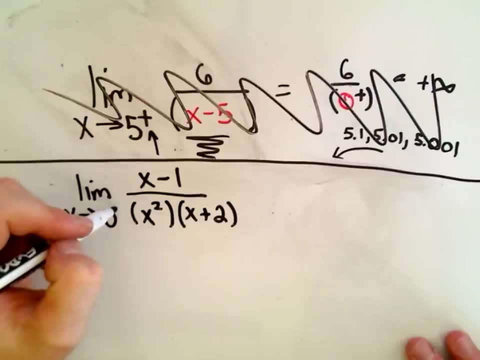 Okay, so I'm going to calculate this limit. Remember, for a limit to exist, the left-hand limit has to equal the right-hand limit. So really, we're going to have to calculate. We're going to have to calculate the limit as x approaches 0 from the left. 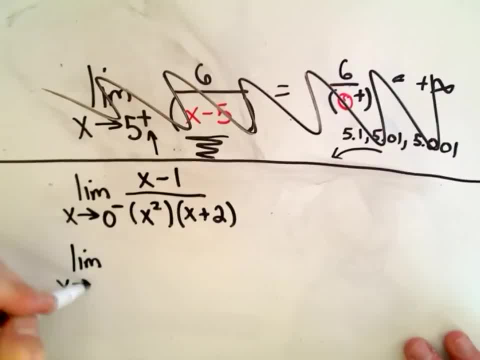 and we're also going to have to calculate the limit as x approaches 0 from the right of this: x minus 1 over x squared times x plus 2.. Okay, so I'm going to do this the same way as before. Notice again, there's nothing to factor in the top. 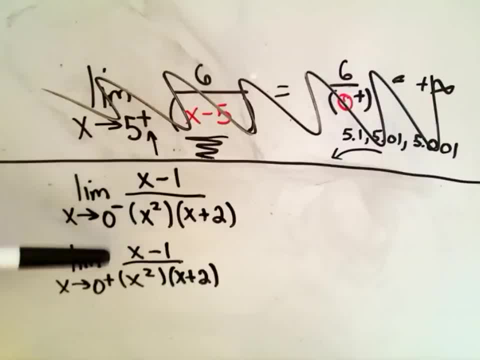 There's no factoring, there's no canceling, and that's something that's important. You want to make sure that things are already reduced and I said that in the very opening. Okay, so I'm going to plug in Again. when we try to do limits, we just try to plug in this value everywhere. 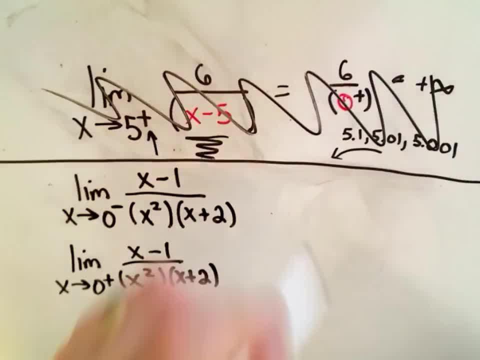 So that's what I'm going to do. I'm going to plug in the number 0.. Okay, on top I get 0 minus 1, which is negative 1.. Okay, fine, I'm not really worried about that at all. 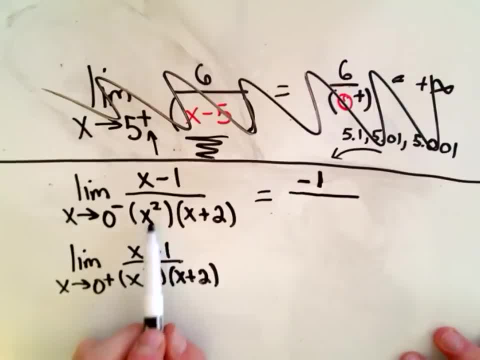 When I plug in 0 in for the x squared, though notice that's the part that if you take 0 and square it well, you get 0. So 0 squared is 0. So that's the part I'm going to have to kind of focus in on and think about here a little bit. 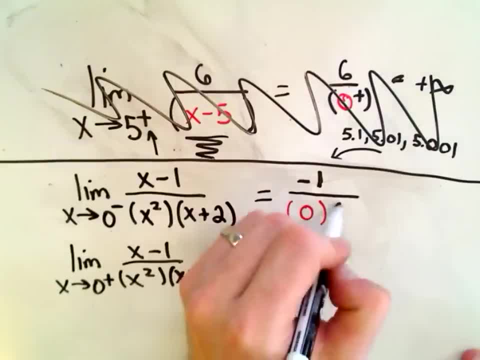 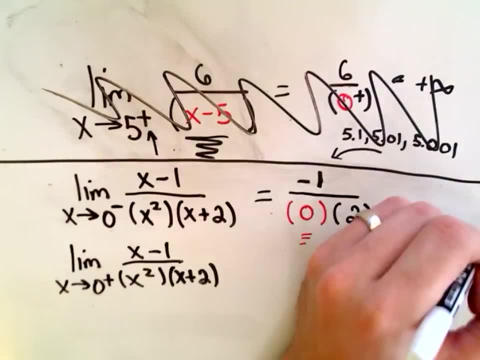 Notice, if I plug 0 into the x plus 2 term, I would simply get 2 out. Okay, and again, I know it's approaching 0 from the left, so that's what the minus means. So here's 0.. 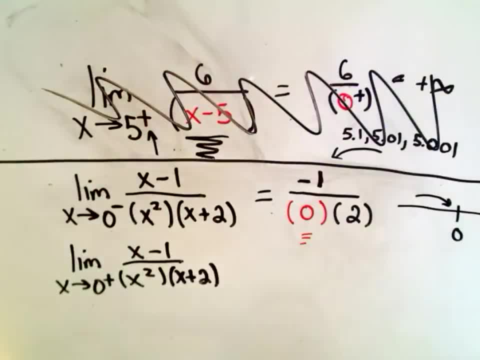 I'm taking numbers a little bit smaller than 0 in this case. So I know that this number wouldn't be quite 2, wouldn't quite be negative 1,, etc. but it would get close to it. Okay, the only thing I have to think about. 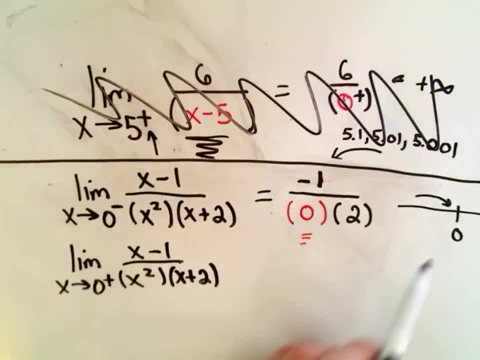 is before the same way. Okay, if I take a number a little bit smaller than 0, say, you know, negative 0.1, negative 0.01, etc. if I were to plug those into the part that's getting squared- well, what type? what would happen to the number? 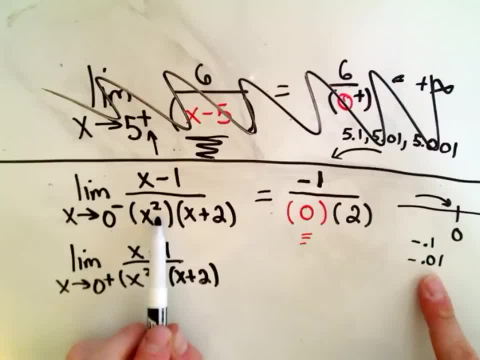 So, since I'm squaring it, it would certainly be positive and it would be even smaller. So when I square the denominator, even though it's a small negative number close to 0,, when I square it it's going to turn into a number that's even closer to 0, but it's positive. 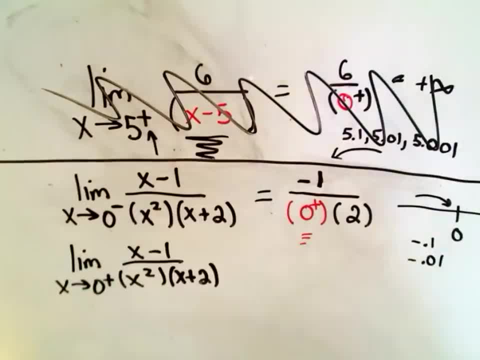 So this would in fact be approaching 0 from the right side. Okay, so again, if you take a number that's close to 0, but negative and square it, it's going to be close to 0,, but it's going to be positive. 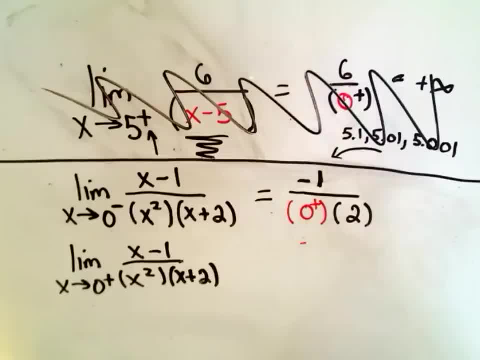 Okay, and now I just kind of do what I did above. I think, okay, on top there's a negative 1. If you multiply 0 and 2, you get 0.. I think about signs: There's a negative, a positive and a positive. 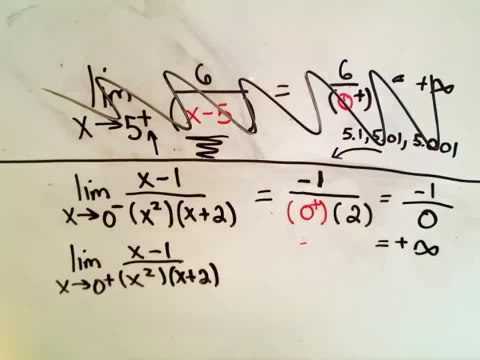 So that's going to turn into positive infinity, Okay, so again I'm being a little sloppy with my notation, So those of you that like to yell at me about notation, feel free to post 80 million comments, But the solution's correct. 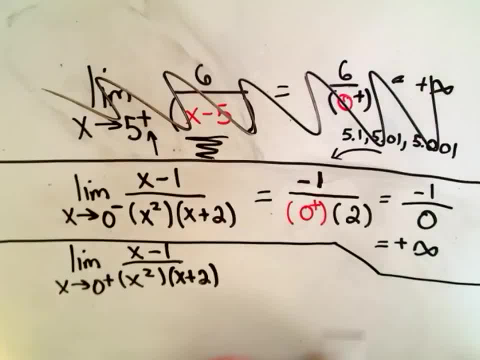 So again, you know, not quite proper notation. I'm just trying to give you really an intuition in how I would think about it in this problem Or in general in these problems. So now we also have to calculate the right-hand limit. 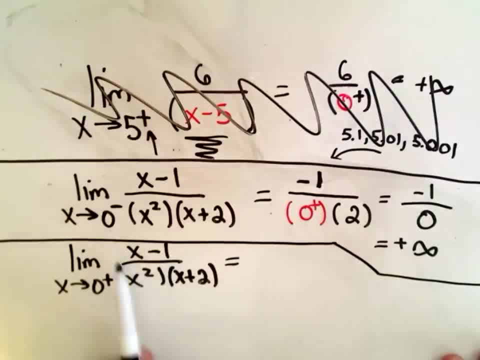 And same process. I think you can see it's going to be quickly, it's going to be the same thing. So if you plug 0 into the top, you're simply going to get negative 1.. Again, if I take a number a little bit, this time to the right of 0. 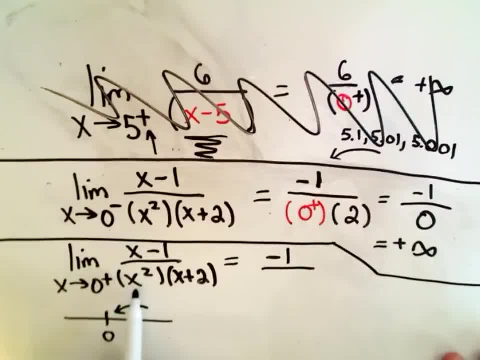 So a little bit to the right of 0. Well, okay, since I'm squaring it, it's going to be a number that's close to 0, but positive, So just like that. And then if I plug 0 in for the x plus 2, you'll get 2..